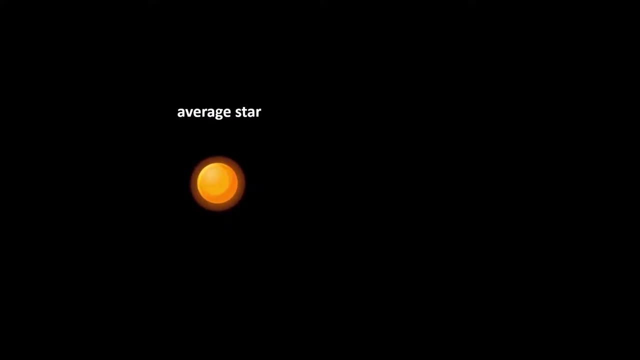 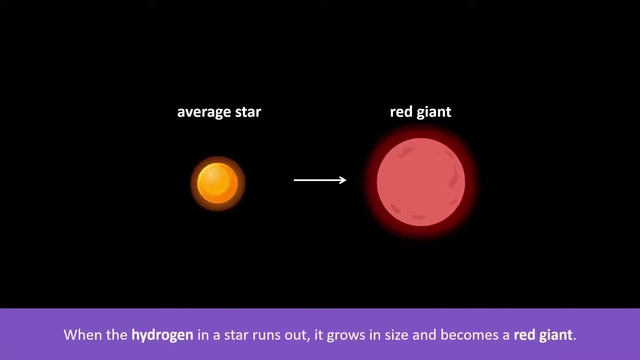 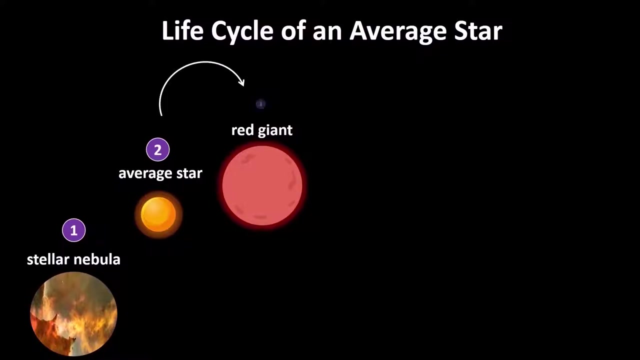 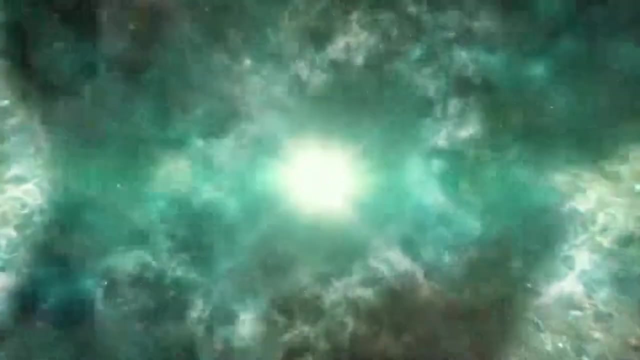 After a few billion years, the hydrogen in the stars runs out. A star then grows in size and becomes a red giant. The red giant will then cool down and begin to lose its mass. Its outer layers will begin to form a planetary nebula. 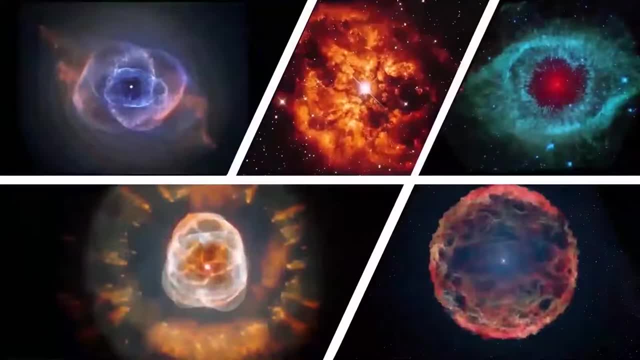 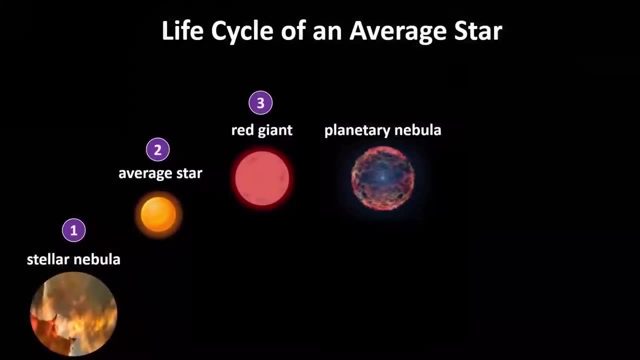 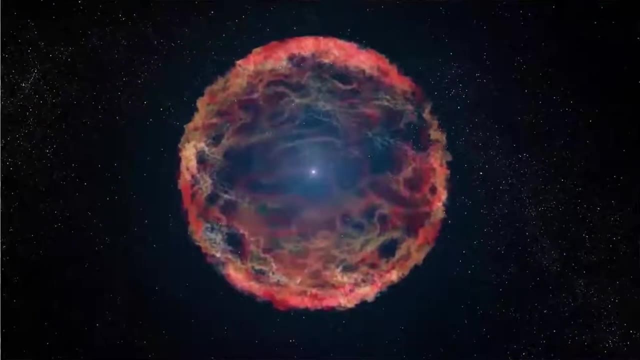 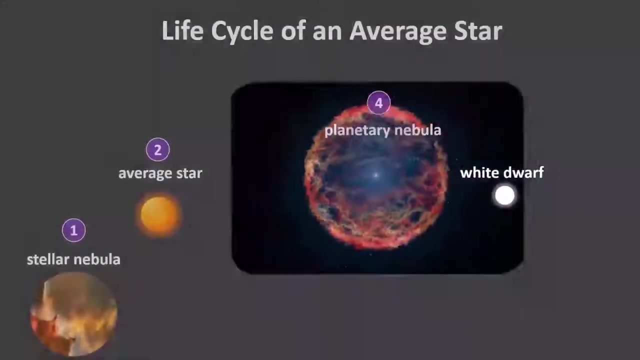 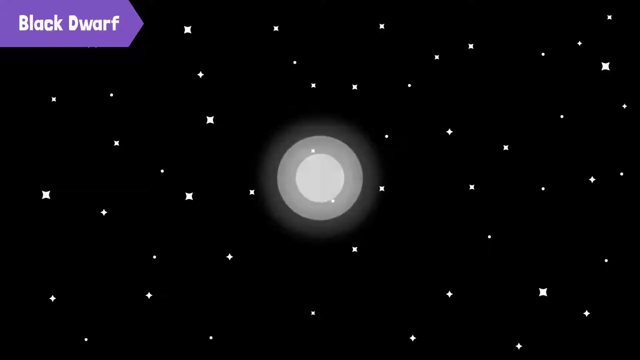 Planetary nebulas are some of the most beautiful objects in the universe. Next, the planetary nebula will disperse, While its core will collapse inward and turn into a white dwarf. Eventually, the star will become a burned out chunk of very dense matter which does not emit light. 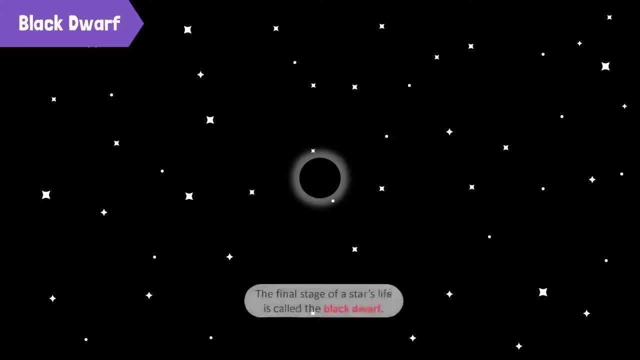 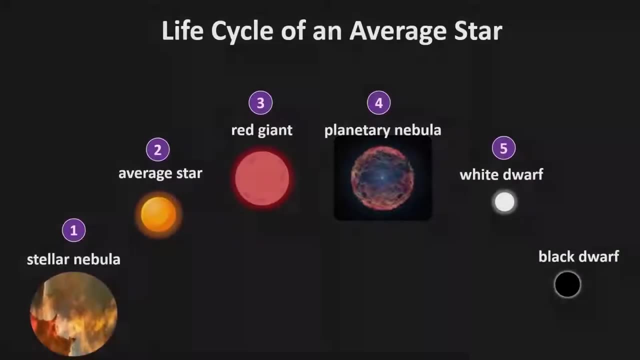 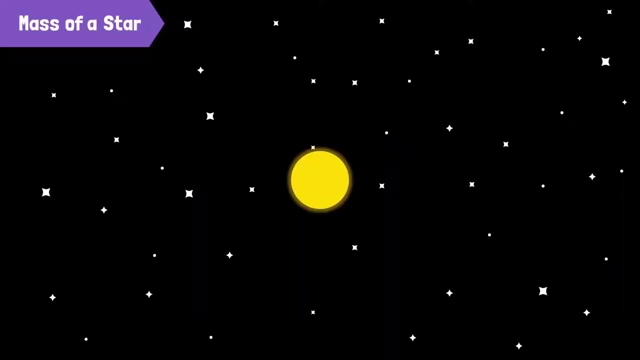 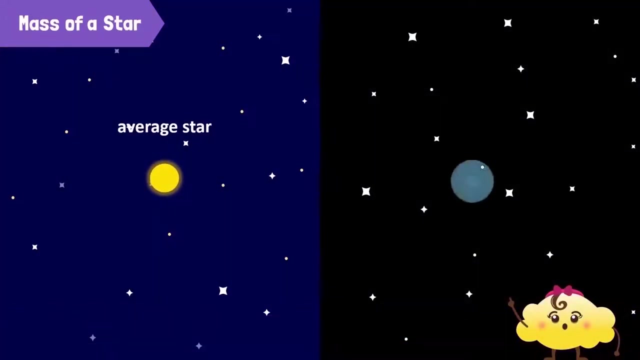 This final stage of a star is called the black dwarf. See, I was right. Not so fast, Spikey. Did you know that the mass of a star determines how it will die? Stars that are at least six times as massive as our sun are called massive stars. 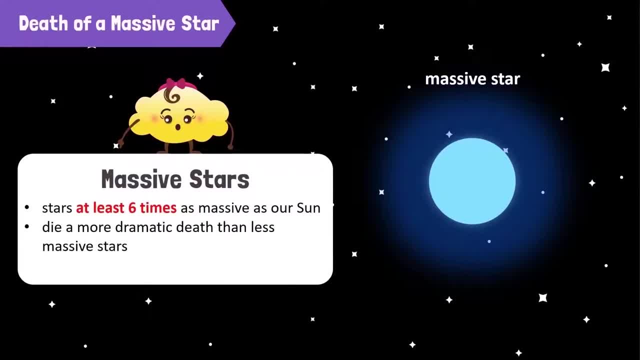 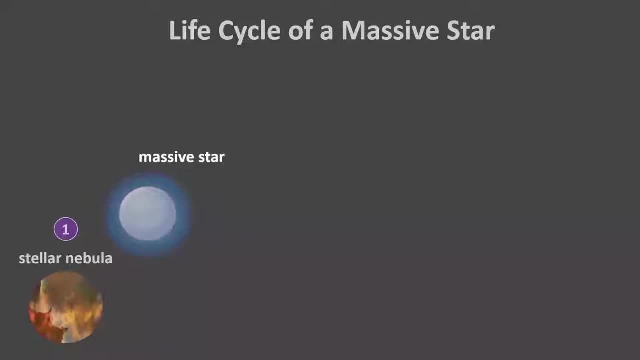 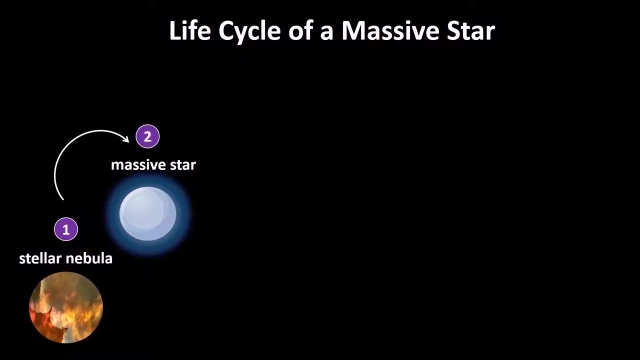 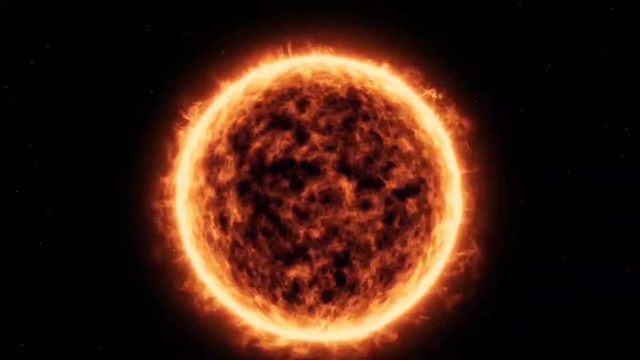 Massive stars die a more dramatic death than less massive stars. They also have a shorter lifespan. Like average stars, massive stars also start out as a stellar nebula. However, their remaining life cycle is different from average stars. When the hydrogen in its core runs out, a massive star increases in size and turns into a red supergiant. 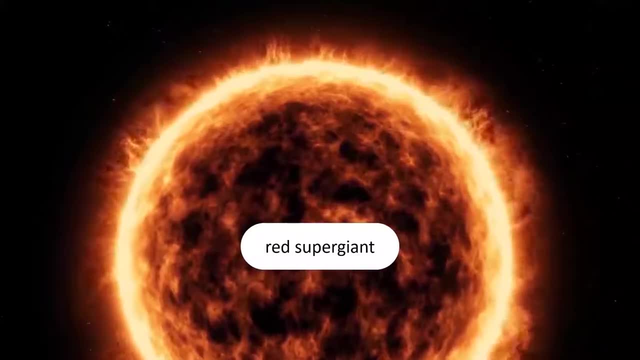 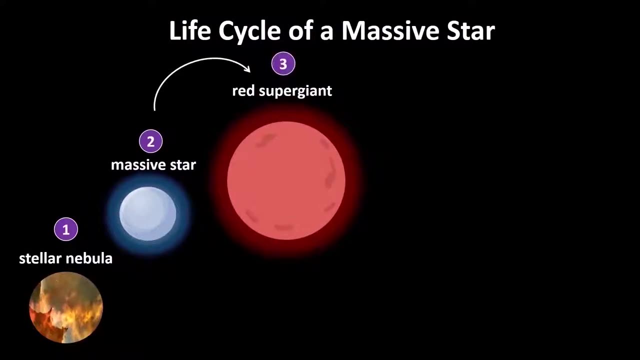 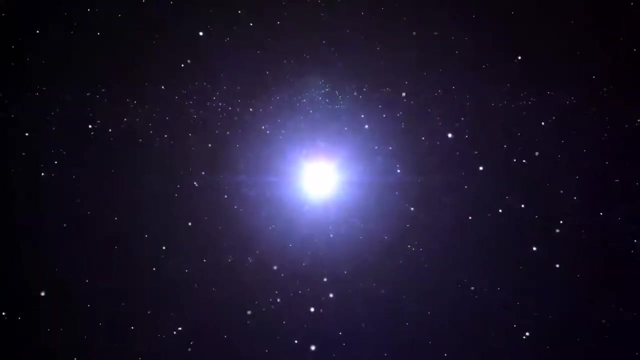 The giant's first life cycle is a total death. They sometimes have a long life cycle, the one in which they can't escape the heat. With time, the supergiant becomes so dense that it crashes inward in a tremendous explosion called the supernova. 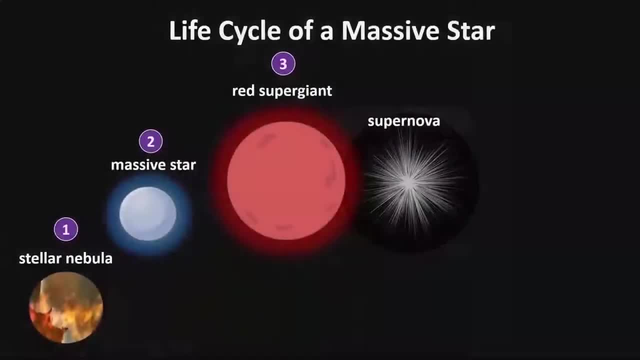 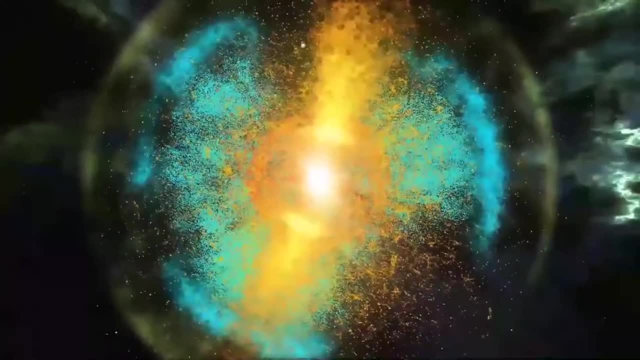 When the current exposes itself in the air, the sun will lose its shape. The energy generated by the hydrogen in the solar plexus is more or less the same At this stage. the light of the supernova explosion outshines all other stars in its galaxy. 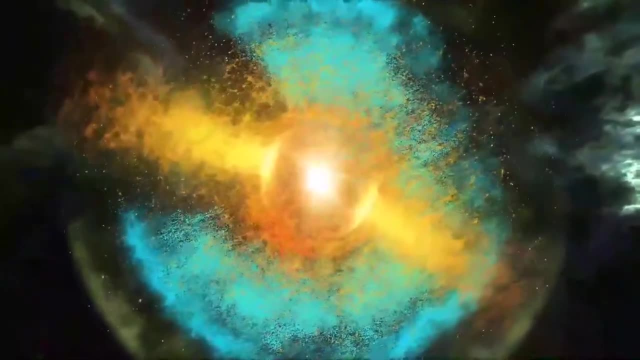 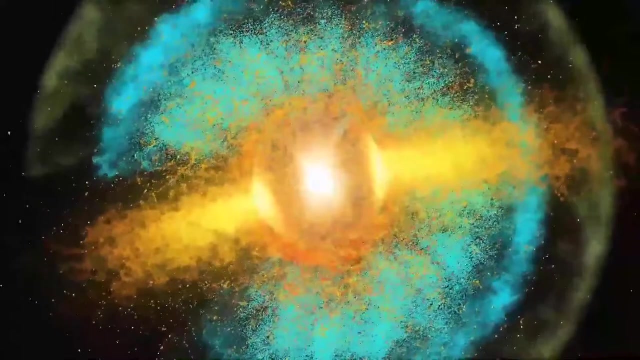 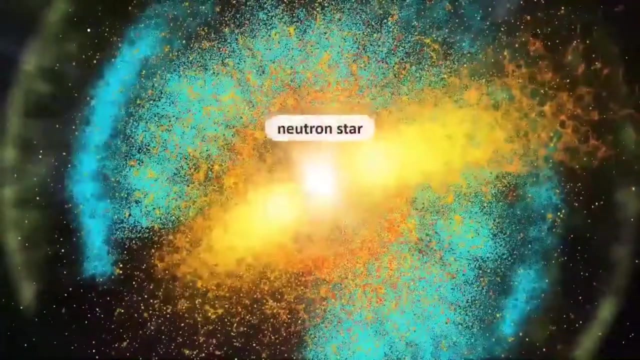 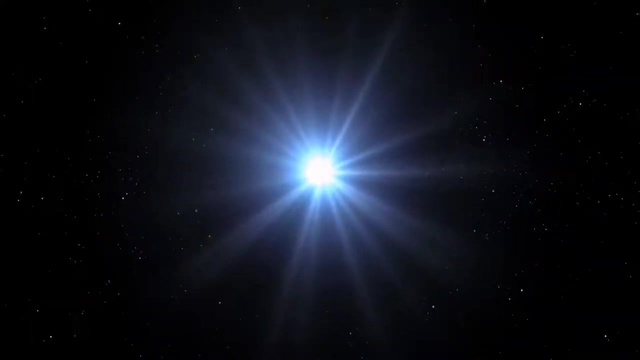 The explosion causes great clouds of gases to fly off the star, leaving behind a super-dense core. This core only contains neutrons, Therefore it is called a neutron star. Sometimes the supernova explosion ends up as a black hole in the universe. 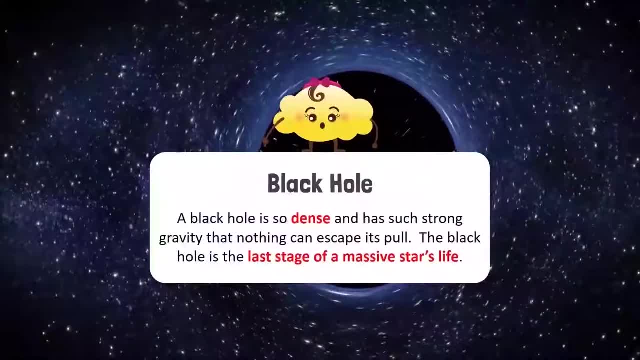 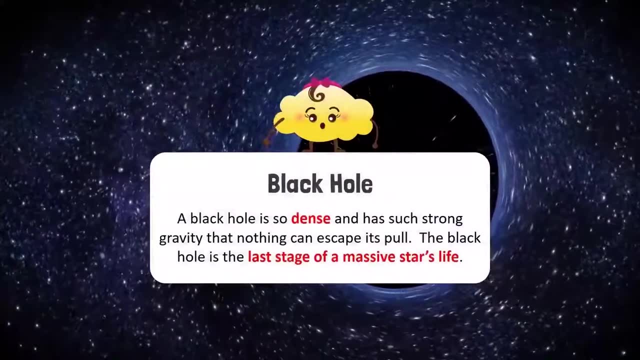 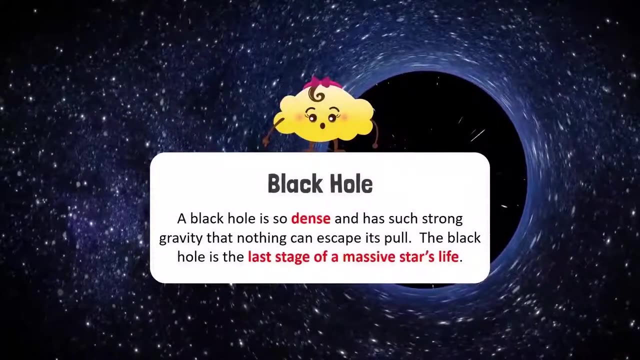 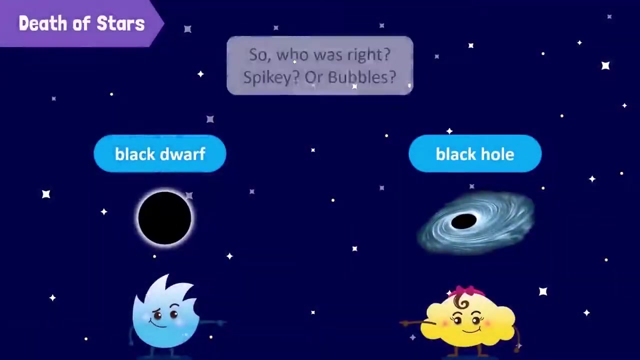 A black hole is so dense and has such strong gravity that nothing can escape its pull. The black hole is the last stage of a massive star life. So who was right, Spikey or Bubbles? Well, both. Spikey was talking about the less massive stars, like our Sun. 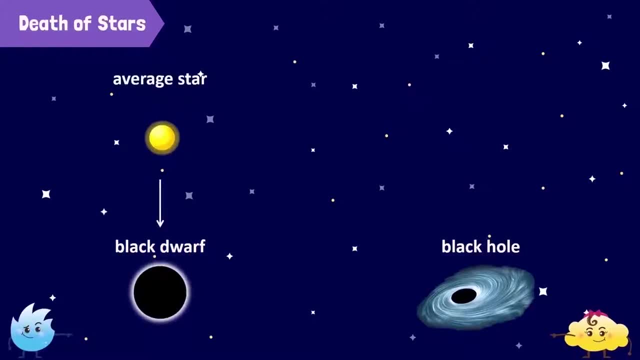 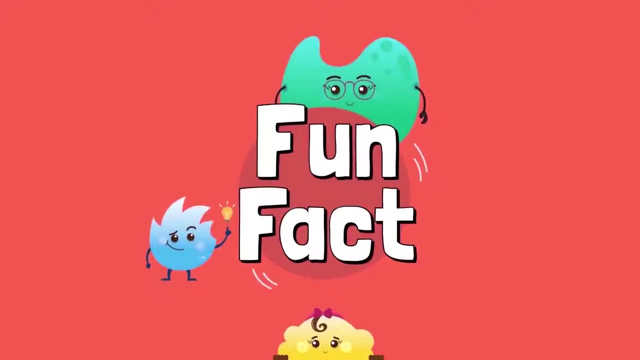 When they die, they'll end up as black dwarves. Bubbles was talking about the massive stars. When they die, some of them will end up as black dwarves. Bubbles was talking about the massive stars. Bubbles was talking about the massive stars. 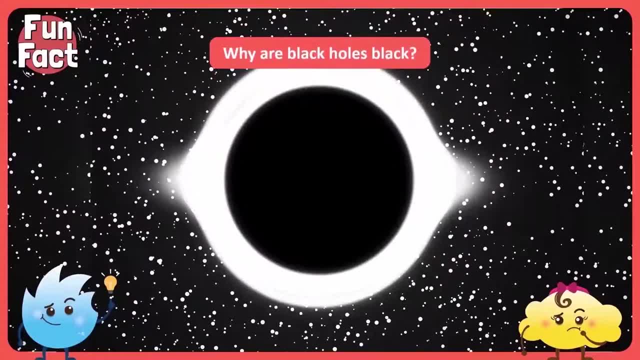 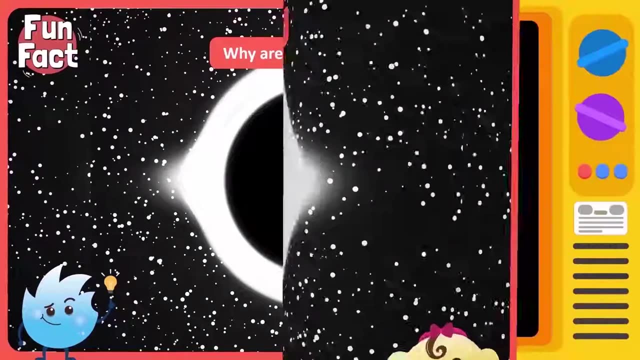 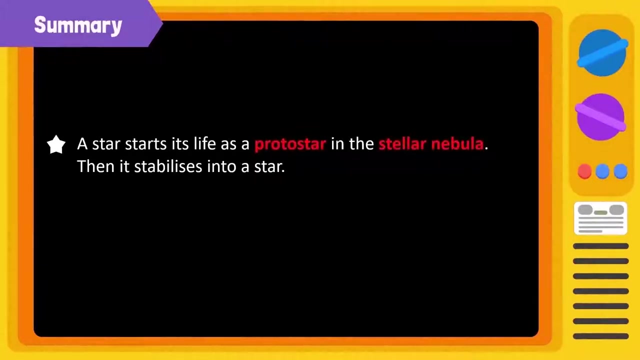 Why are black holes black? Black holes are so dense that nothing can escape their pull. Even light cannot escape a black hole. This is why they appear black. Let's summarise: A star starts its life as a protostar in the stellar nebula. 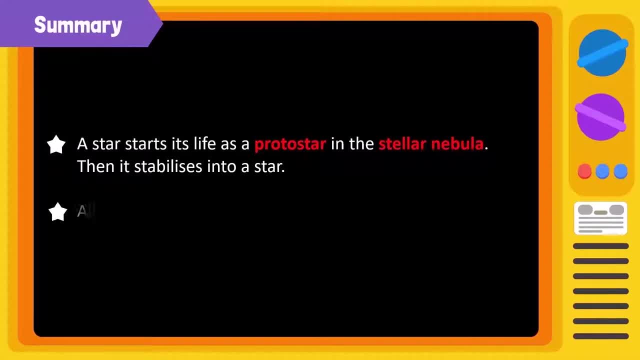 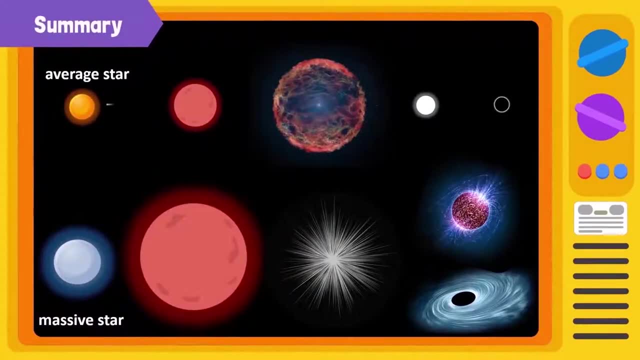 Then it stabilizes into a star. All stars are born the same way, but die differently. After exhausting its energy, an average-sized star becomes a red giant, then a white dwarf and then dies as a black dwarf. A massive star has a different journey.